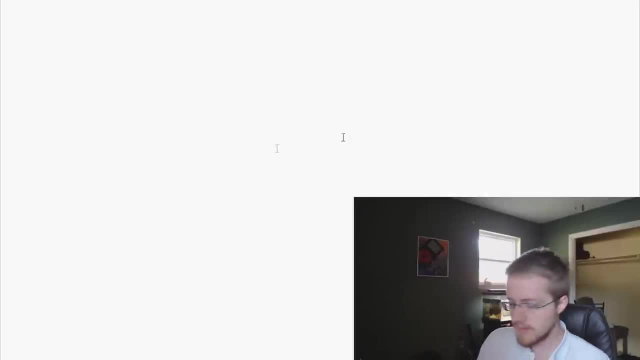 Kind of like global modules. So with that, let's go ahead and get started. The first thing that we want to do is we want to go ahead and make a simple module that we can use as an example. So let's go ahead and do that. So, as we've kind of shown before, a module is just a Python script usually. So that's it. So what we're going to do is just make a simple script and we're going to say: define example or ex, and ex is going to have one parameter and that's going to be data. Now, all this function is going to do is 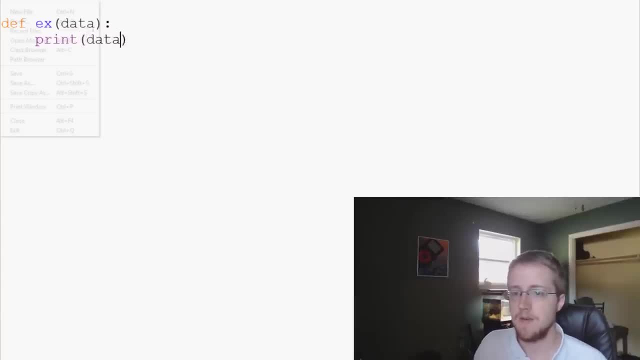 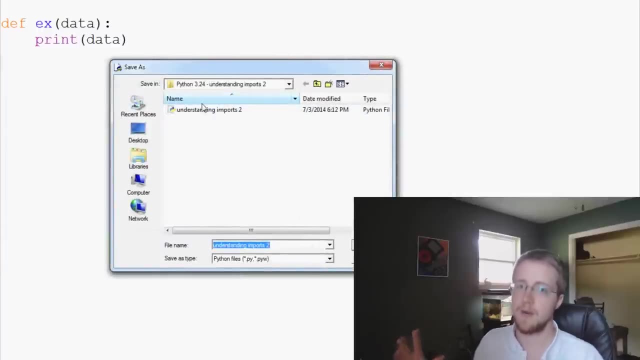 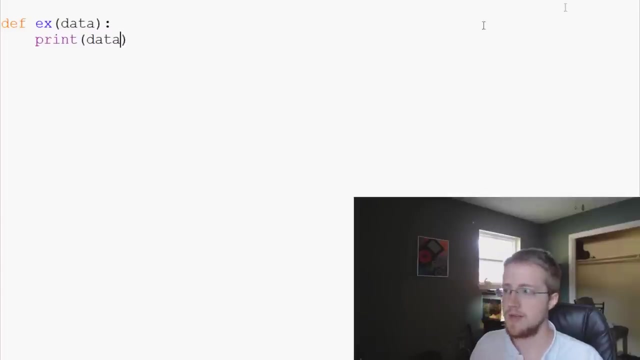 it's going to print data. That's it. So now we're going to go to file, save as. and we're going to save this function in the same directory as the current script that we're writing And I'm going to save it as example: mod dot, pi. Save that and we're done. Now we can open up the original script, which should be empty still. Come back over here, Make it the proper size. And now we're going to 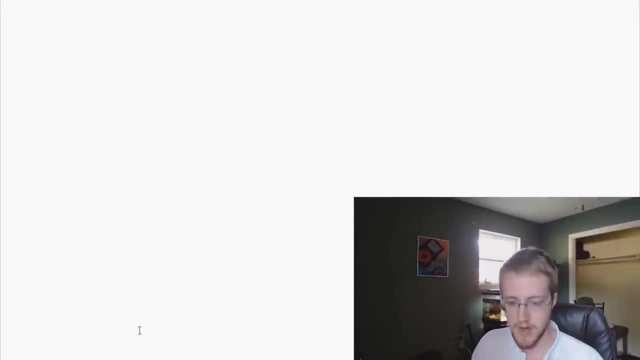 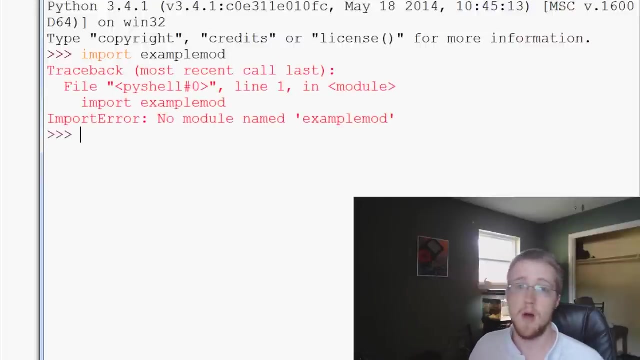 ready to maybe use this module Now, just real quick, we can go start and what we want to do is we want to open up a Python 3.4 IDLE. And real quick, let's just try to import example mod. We get an error and it says there's no module named example mod. Basically, the path that it's going to go through to look for modules is going to be like local site packages and lib, Right. So see Python 3.4 lib. See Python 3.4 lib. 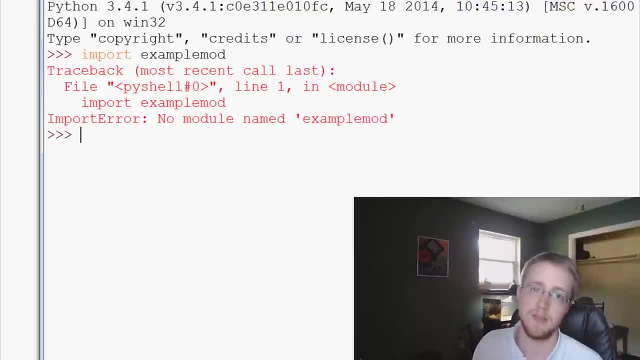 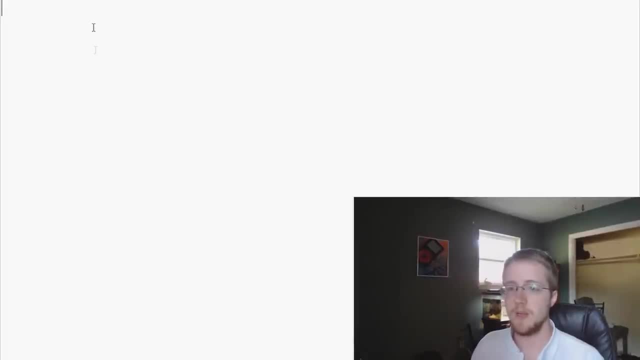 Generally, again, third party modules will be inside packages, whereas your typical vanilla installation modules will be right there in lib. So with that, we can come over here, though, and we can go import example mod and, just real quick, let's save and run it, And we see that we don't actually get an error. Okay, And that's because we do have it. It's local Right, So it is in one of the checking, checked paths. So now what we can do is we could actually say it from: Well, we have an import example mod. 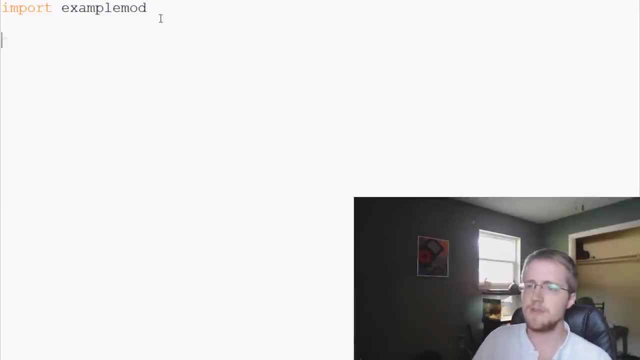 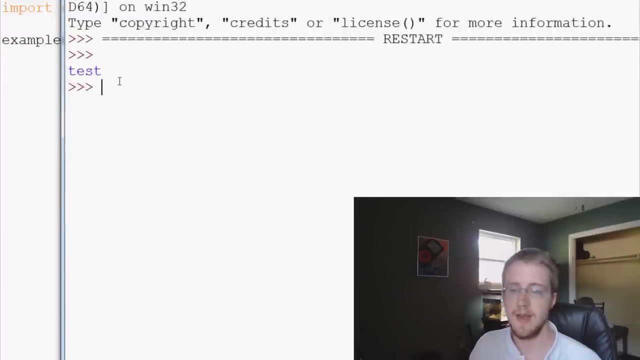 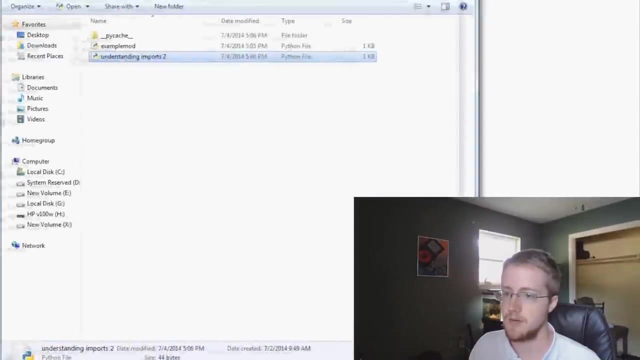 Now, as we showed in the last video, we still have to do something like this, like example mod, dot e, x. And then in here is where we're going to put our data. for us Let's just say test. So it should just print out test. So we'll save, We'll run that And, sure enough, the output is test. Now we can take this a little step further and we can go into the directory that contains our script, which is here. So we have example mod. Now we can do is go my computer here, See. 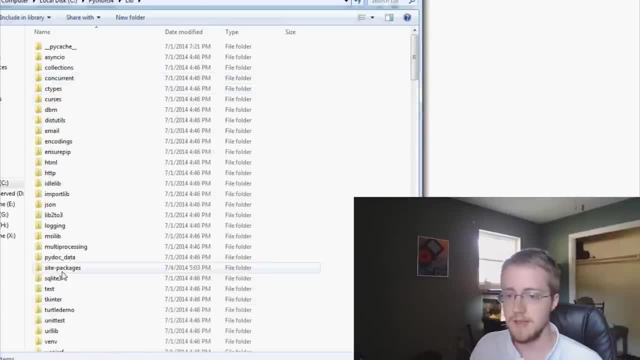 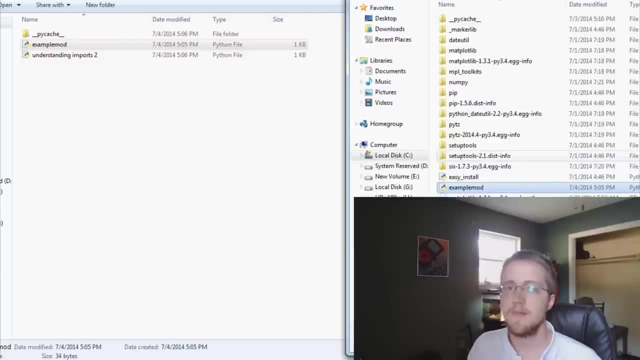 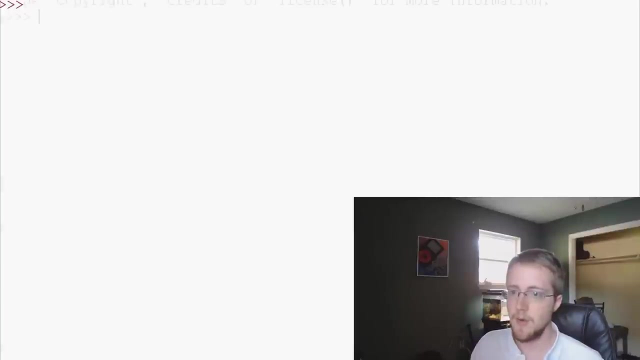 three, four lib site packages. And now let's go ahead and just copy this module into site packages. So now we have example mod in there. So if we go again to our Python three, four, IDLE, What we can do now is import example mod. And now we can go example mod dot e x test And it acts as any other. 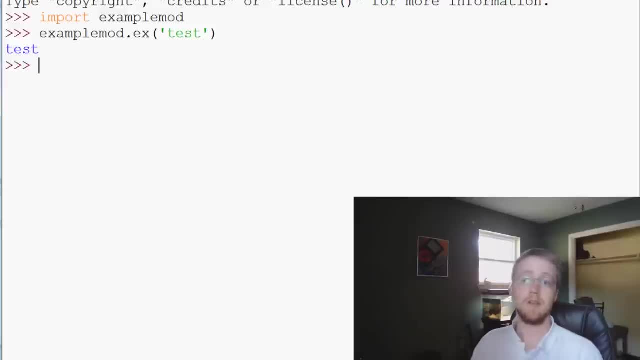 module would act. So that's how you can kind of create your own modules and you can obviously edit modules. And if you do create your own modules and it says it doesn't exist, Well, it needs to be in one of the paths: local lib, site packages, OK, And that's pretty much it. And so what you can do eventually is download, like, say, you're going to say you make your own script that you find extremely useful and you find yourself using it every time. Let's say, you like, for me, I do send them an analysis and a lot of times I use the same part of the. 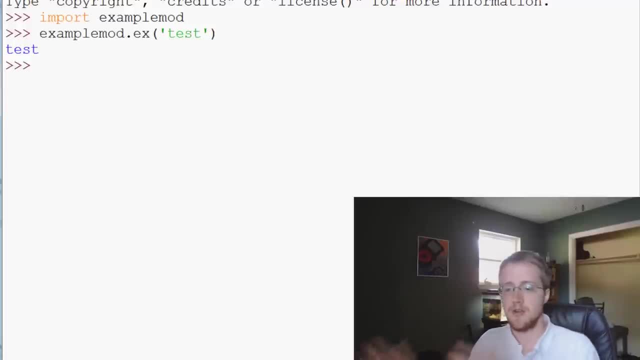 parser for no matter what the website is, I use a parser and then I usually apply some rules to it and all that. I'm going to put that in my site packages because I use it all the time. So why not just import that? instead of, for every kind of application that I use a parser for, Why not use the one that I've trained really well? So, anyway, that's just an example. You'll probably have your own, But that's so you can make your own modules. Also, if you download someone else's module, or maybe you see someone else's code that you want to make into a module yourself, and they don't necessarily have a set of modules.